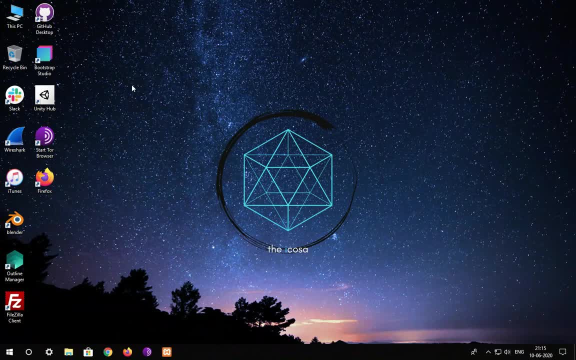 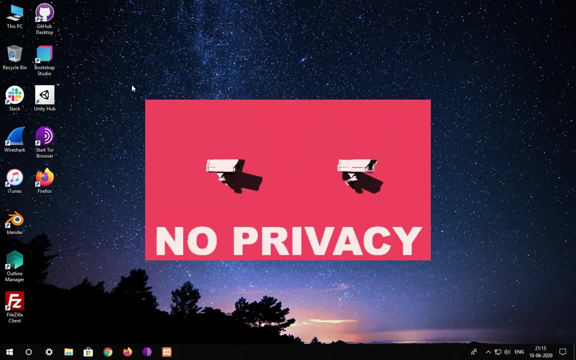 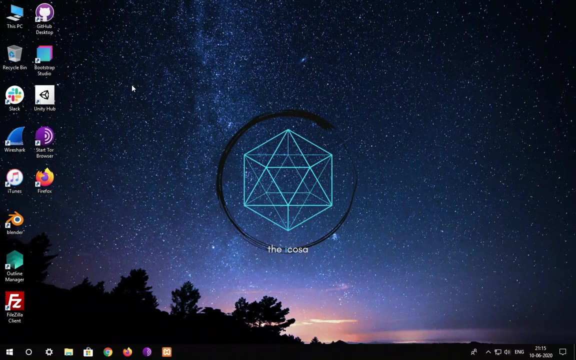 But you know what? Even the incognito search is not sufficient if we really are concerned about our privacy, because Google is even tracking the incognito. It's like it's not just that, even if we just clear the history, or the history isn't saved. 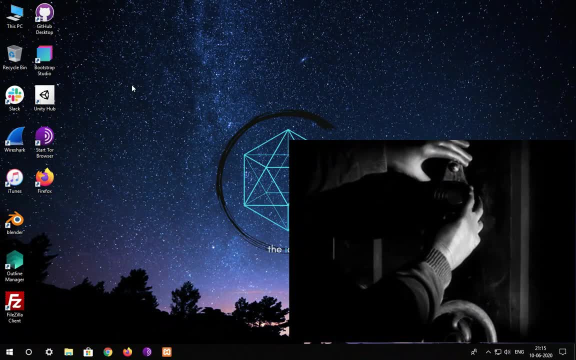 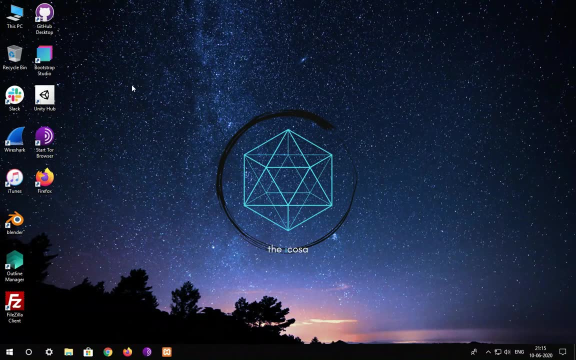 that doesn't mean that someone is just not tracking us. You know That If you are watching this video on YouTube, Google knows that you are watching this video- and like, if they tomorrow, if they want to see that who people who are, who were the? 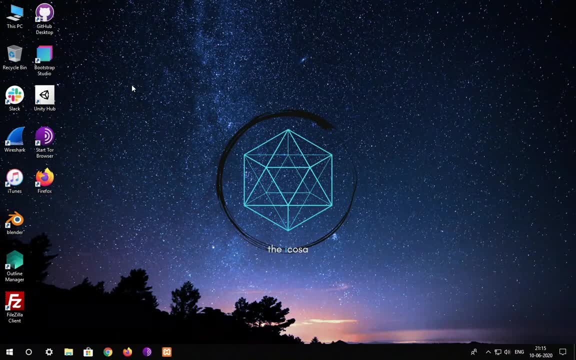 people who were like watching this video yesterday. they can just take that list out and they can point you out right at the moment. So the question is: how do you stay safe, How do you stay secure when you access the internet? Well, 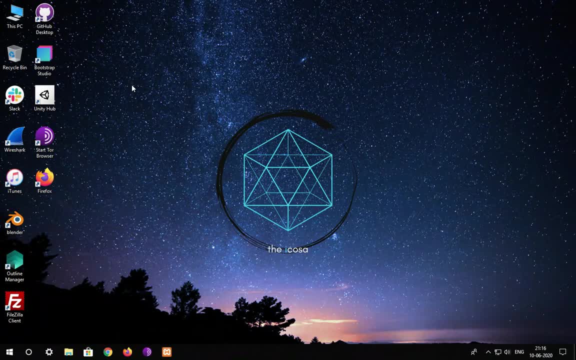 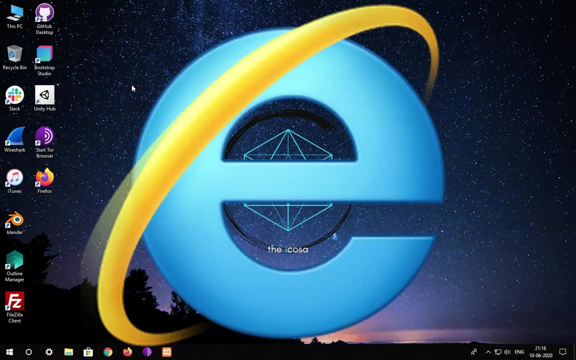 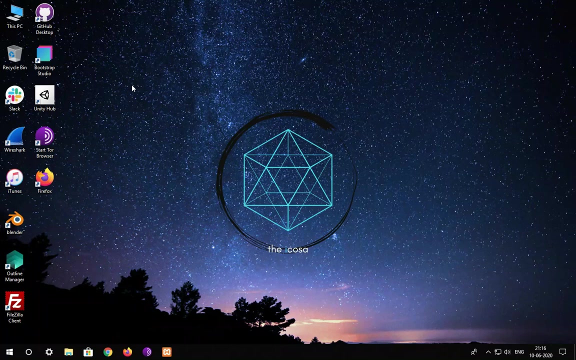 There are some good companies who have made browsers which search the web even better than Google. Yes, Even better than Google, even better than Opera and even better than Internet Explorer. Yes, I'm right, Internet Explorer. I don't know who uses it, but yes, Internet Explorer as well. 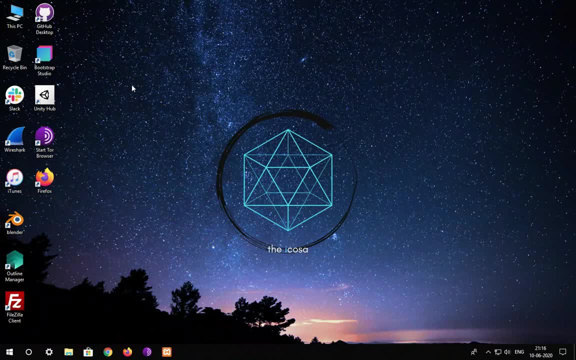 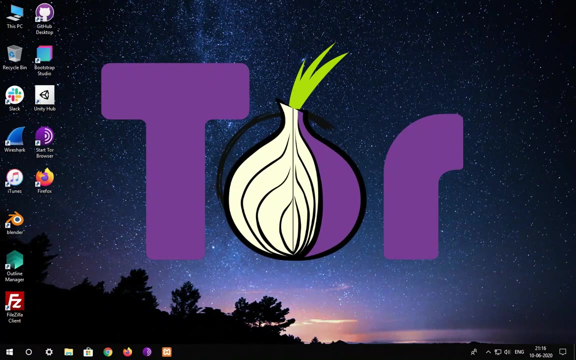 So what's the name of this browser? Well, The name of this browser, The name of this browser is The Onion Router. Yes, The Onion Router, or simply Tor. Yes, T-O-R or The Onion Router, That's the name. 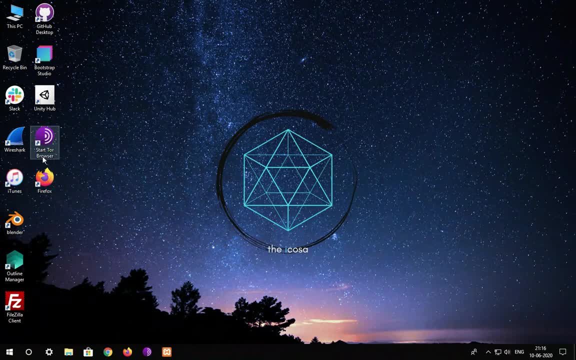 Okay, So I have this thing over in here, like, say, it says Start Tor Browser, but, but, but, but, but. but how to install it? where to find it? Well, let's head on to Google Chrome and I'll teach you that where to find it. how to find. 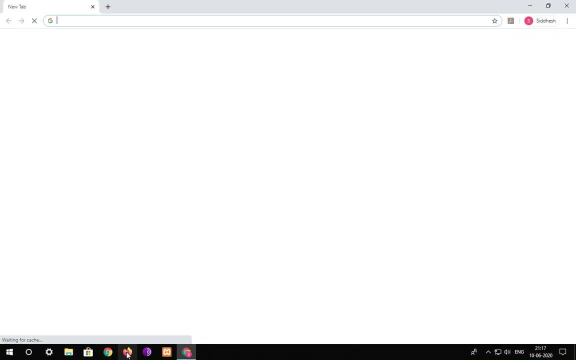 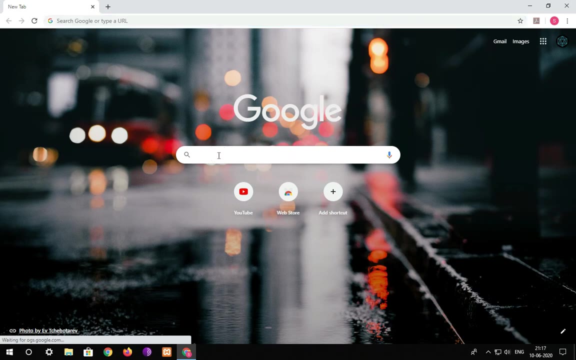 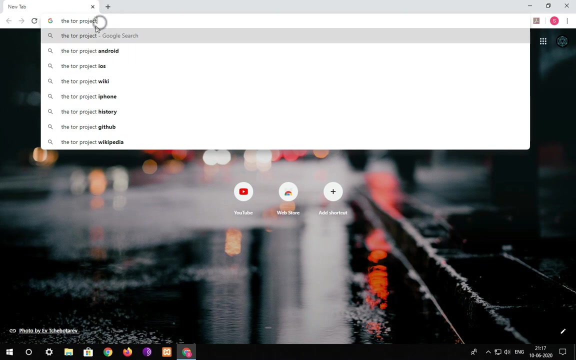 it. Okay, So just go on and open Chrome. Yes, You can open up Firefox as well, or Internet Explorer, if you are really using it. Okay, So let's go on and type in the Tor Project. Actually, this is the thing which you need to type in, or you can just go on and type. 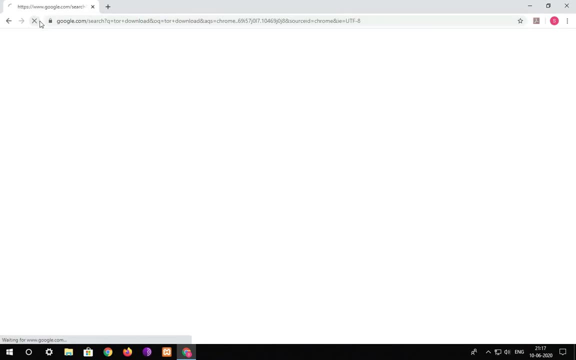 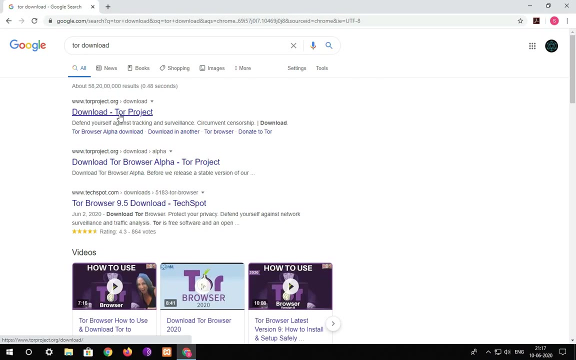 in like Tor, Tor Download, And the first thing over here is the wwwtorprojectorg, which is the official site of Tor Browser, The official site of The Onion Router Browser. Okay So, but but before we install this, we need something else as well. 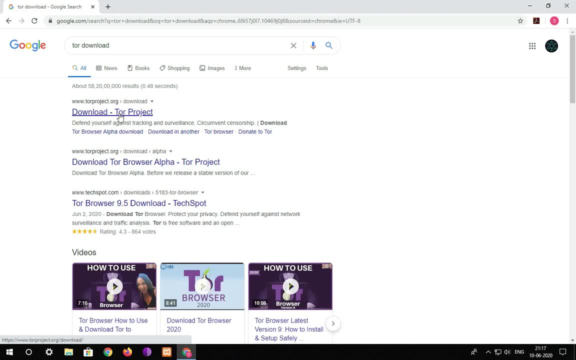 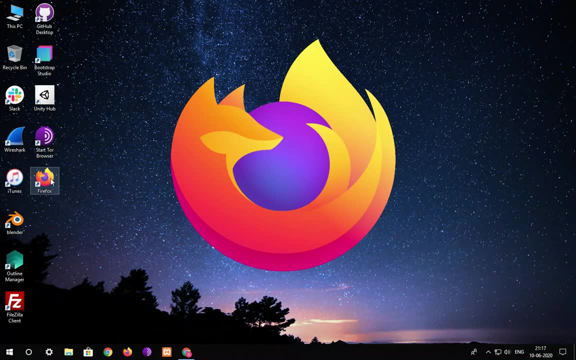 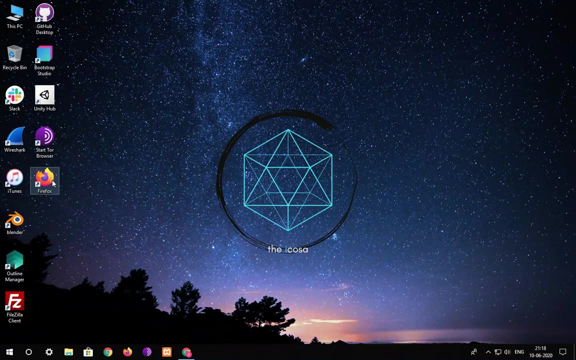 Okay, And what's that? Well, it's this thing over here. Let me just show this to you: Firefox. Yes, And why? Because Tor, or The Onion Router, actually runs on Firefox, So it's simple to install it. 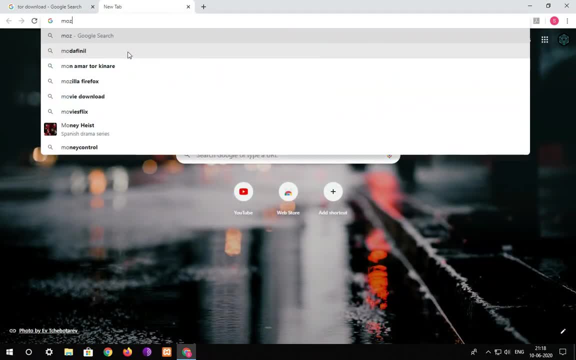 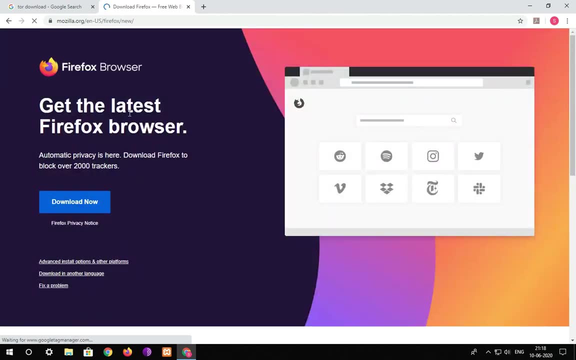 If you haven't really installed it, just go on and type in like Mozilla Firefox And you get the download link in here. Just go on to it And it's in here. Just go on or go below. Okay, So that's the link. 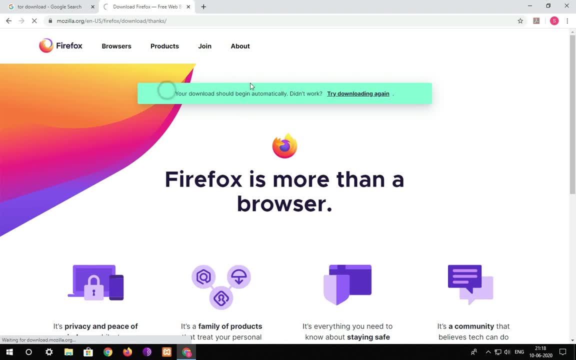 Fine, Download now And the download should start automatically. Yes, it's in here And okay. so this is the setup. You can just go on and open it and run it And it will start this thing Now I have already installed it. 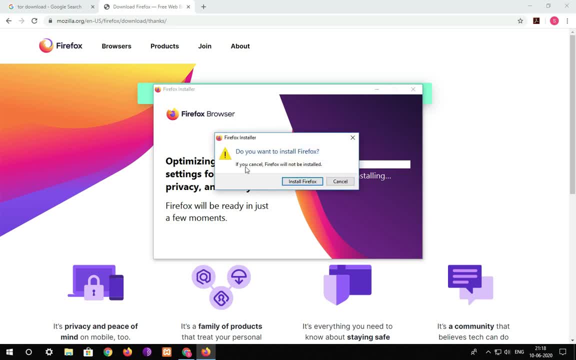 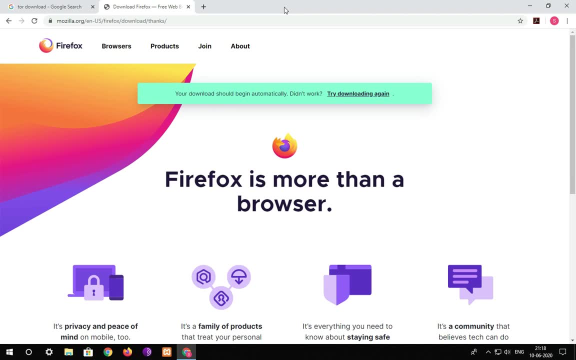 So I just won't install it. Yeah, If we cancel Firefox will now. Yeah, Fine, Fine, Fine, Cancel that. Yes, I know the download was interrupted because I already have downloaded that. Alright, So after we have downloaded Firefox, 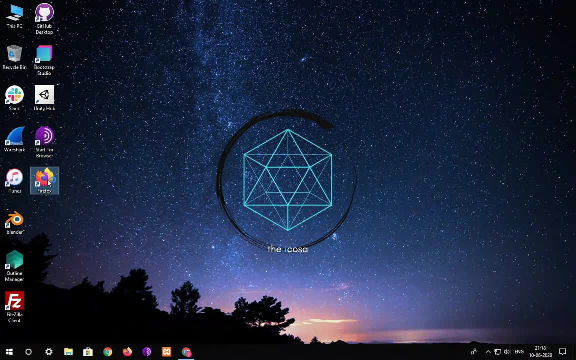 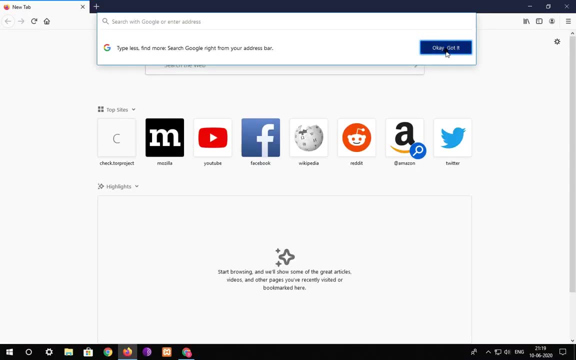 Firefox, Sorry. So just check it And if it's working, I'll just open it up. Okay, I got that. Okay, So this is the thing And this is how Firefox looks. Tada, Well, that was all. 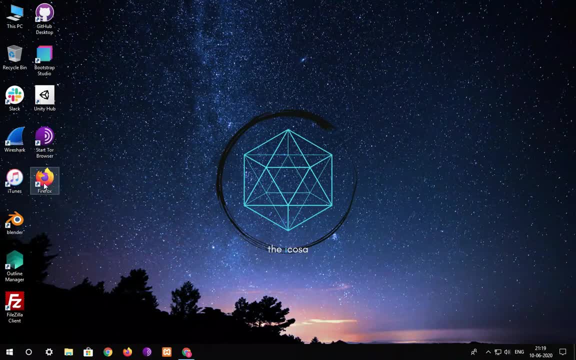 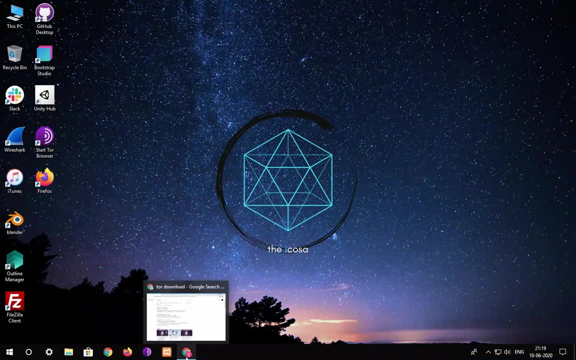 Fine, Just close this in. Okay, Now, after you have downloaded Firefox. Firefox, I'm really sorry, I'm just misspeaking it. Sorry for that. So, after you have downloaded Firefox, just go on and you can see this thing over here. 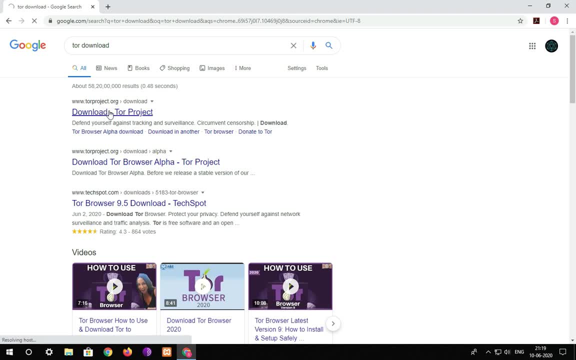 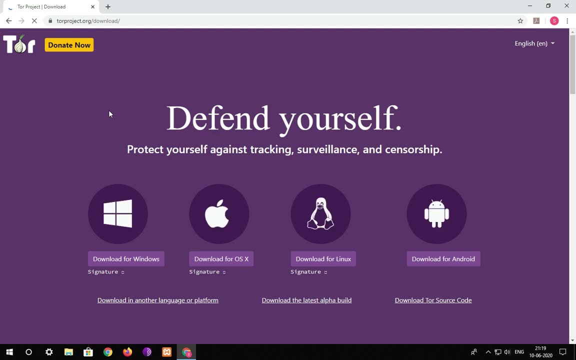 Download the cloud project. Just click on this So it will start. Sorry for the slow internet connection. It's really slow. Sorry for that. Okay, So here you can see. it works on Windows, Apple, Linux and Android as well. 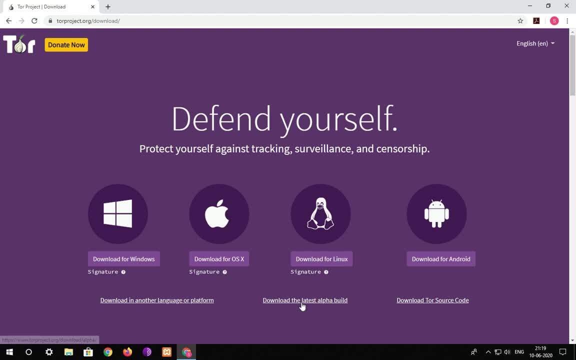 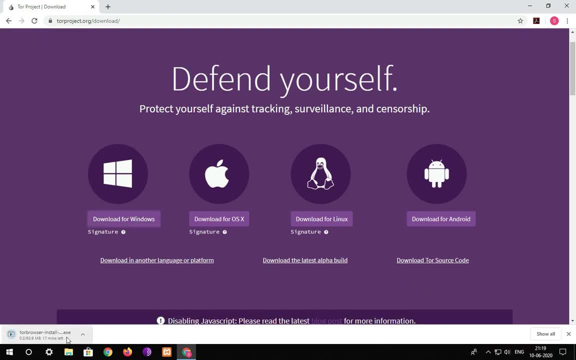 Yeah, I'm really excited for this, But for now, as I'm using the Windows operating system, just go on and download this thing. Okay, So this is just the Tor setup And I have really installed that. So I just won't download that again and again. 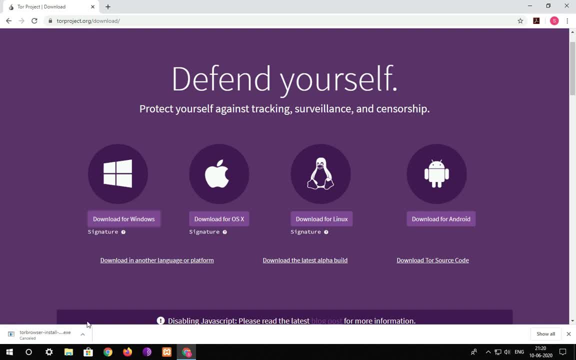 I don't want to waste my data, Sorry for that. Okay, So after you have downloaded the Tor browser, you just need to like install it like a normal software. So just click on that, Run the software and install it in your C drive or whatever drive you've installed it. 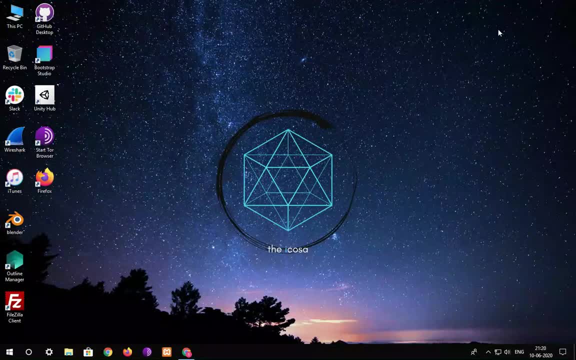 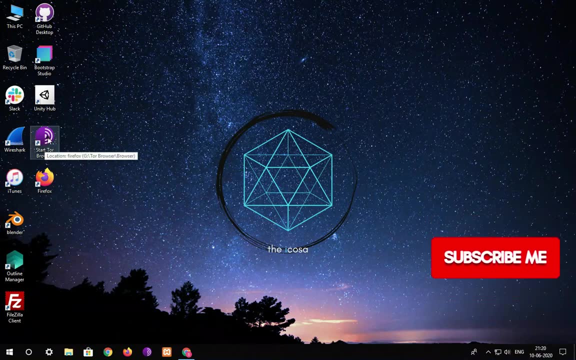 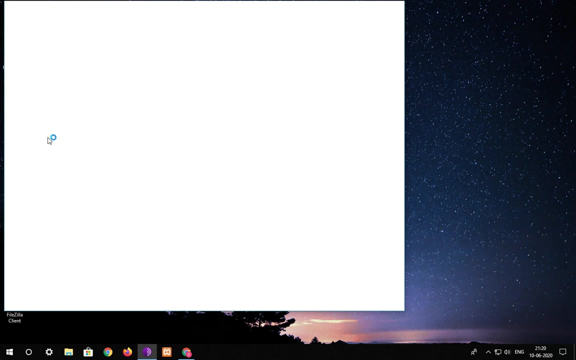 in Now, what after that? Well, I'm here to explain you that Now. just, you'll get this thing over here. It's a desktop shortcut, So just go on and double click on this thing. Okay And yeah. 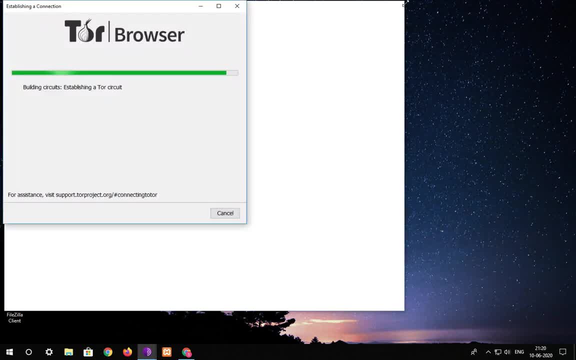 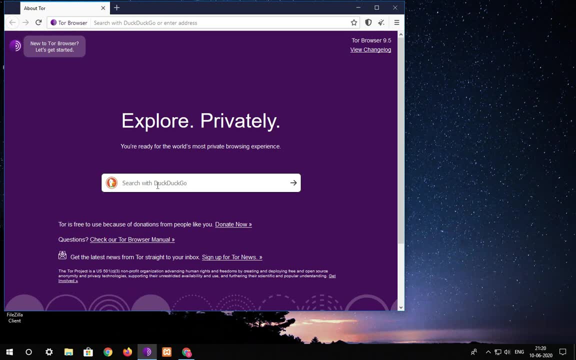 One thing, One thing for sure: If this opens in such a window, just let it be that way. Okay, And the first thing is that it won't give you this window. It will give you something like this, which appeared over here: 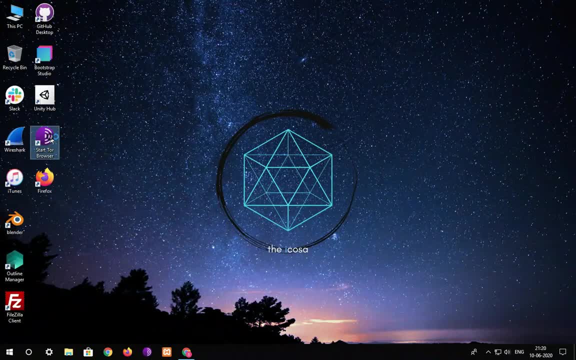 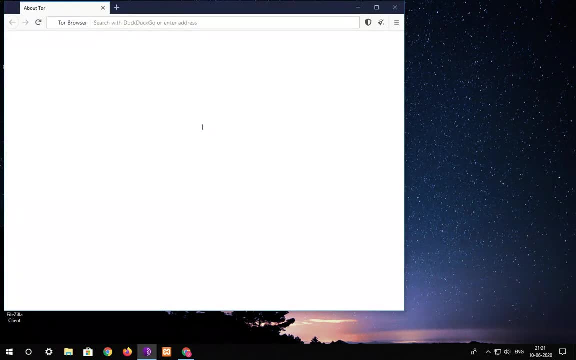 The box over in here. I'll just close this and open it again. I'll tell you what thing will come up the first. Okay, So this thing will actually come up the first and you'll get two buttons over here. First one will be connect. 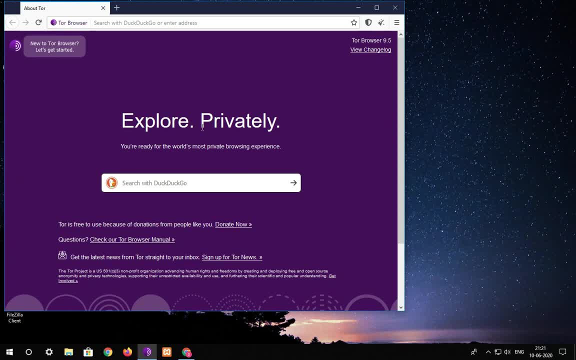 And the second one. I don't remember that. what was what? So just click on the connect button and you'll be prompted over here, Alright? So what do we do now? Well, you have done everything. Yeah, I mean just literally everything. 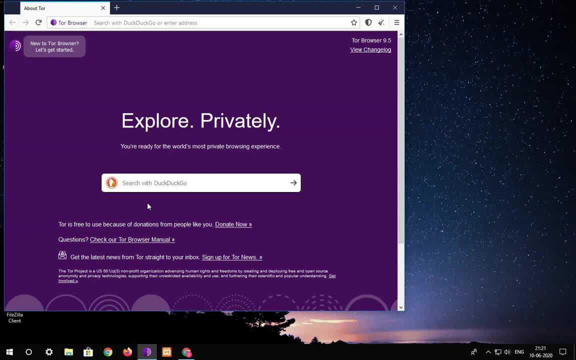 That was all. Just install the Tor browser and you're ready to explore everything privately. Now, how do you know that it's installed and it's really working? Why You don't trust me? huh, Well, fine, No problem. 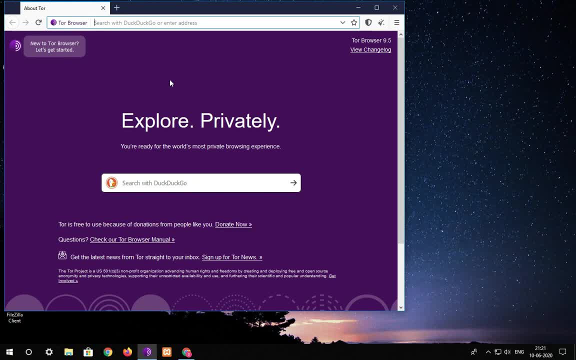 Just go on and search in here. Now, the thing which we'll notice over here is that it uses the DuckDuckGo search engine, which is actually pretty awesome, because Google hides many things from the search engine, like it goes on hiding things, like I won't say that, but it hides many things, just like torrent. 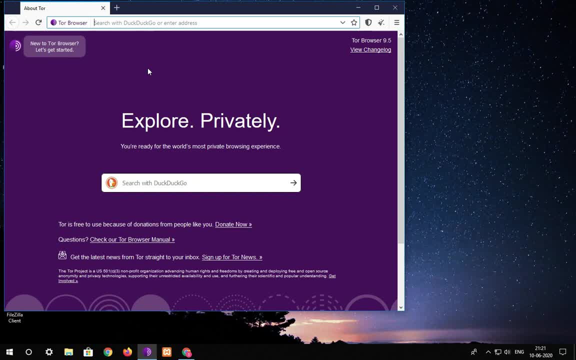 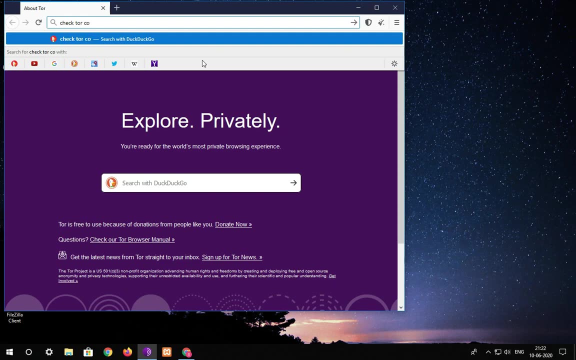 links and some explicit content which I'd not like to tell. But that's the way, So just go on, and it's actually really reliable. the DuckDuckGo search engine: I really trust that. Okay, So just go on and type in check or connection and hit enter. 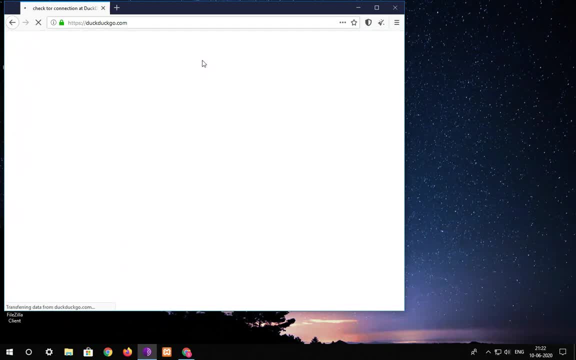 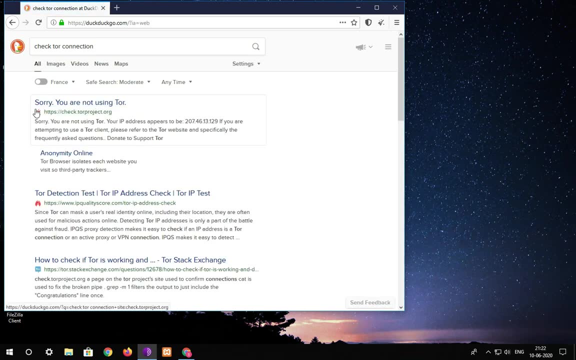 And there we go: Ooh, la, la, Okay, So you'll see this page. Yeah, I know it says sorry You are not using Tor, but fine, When we open that link, we'll surely get that. Now, before I open that link, let me tell you something. 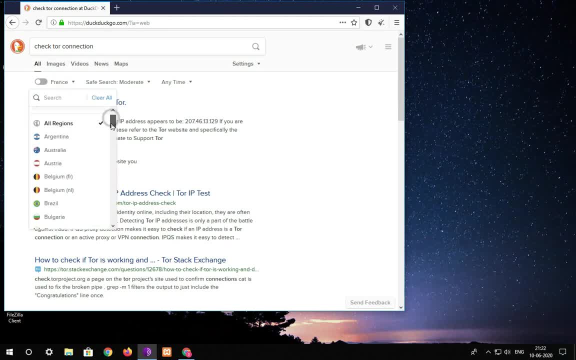 You can see this thing over here, right, It's like an inbuilt VPN which you can actually connect, Okay, And this thing is really really, really awesome, Okay. So it's like our regions, and then Canada, China, India and United States and this stuff. 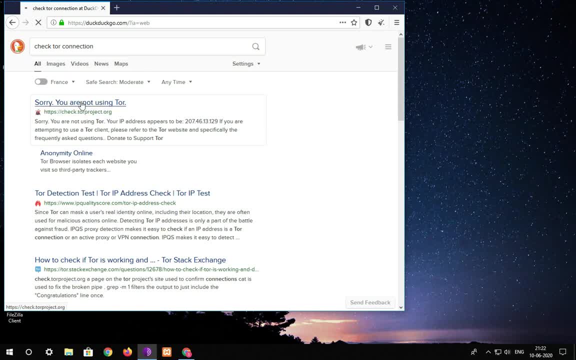 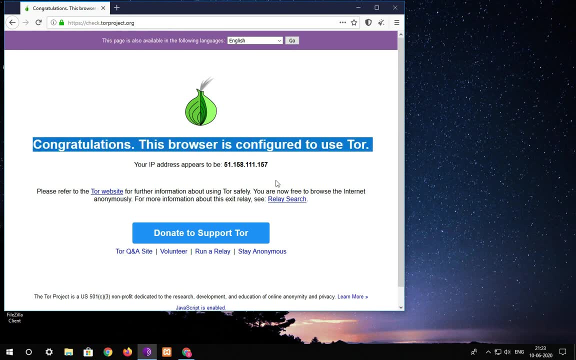 It doesn't stop. It just covers many of the countries. Okay, So I'll just click on this thing. Okay, Fine, And after you click on it, you'll get this thing as congratulations. this browser is configured to use Tor. 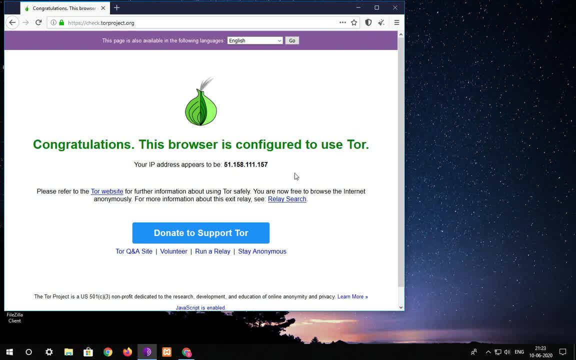 Yeah, And this simply means that you are using an anonymous network which is called the Tor. It actually says that you've connected to the Tor network, which is the onion router network. Fine, Now let me show you some proof. Okay, So just get back. 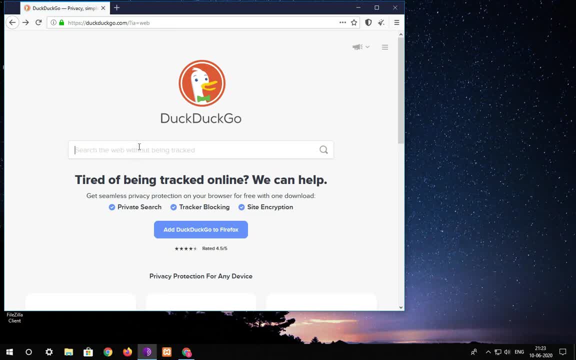 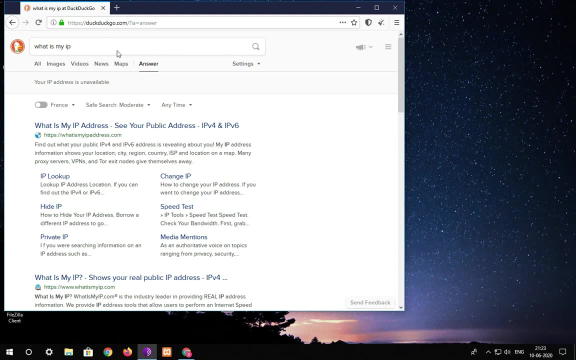 So just get back in here and like, okay, I don't want that, I don't want that, Please. Okay, And I'll type in, like: what is my IP? Well, for the people who don't know what is IP, IP is actually an address which is located. 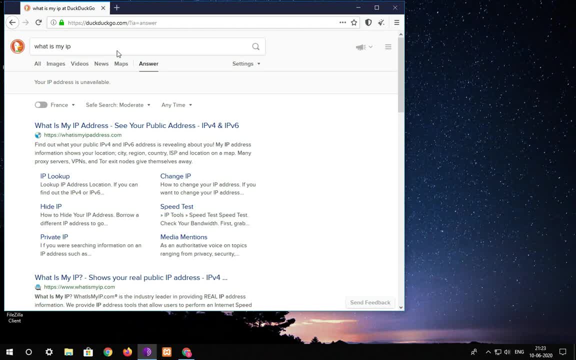 to your computer. It's like, let's say, you have a home address In the same way you have a computer address as well, And that's all what you should know right now. I'll be having, or I'll be making videos on that later on as well. 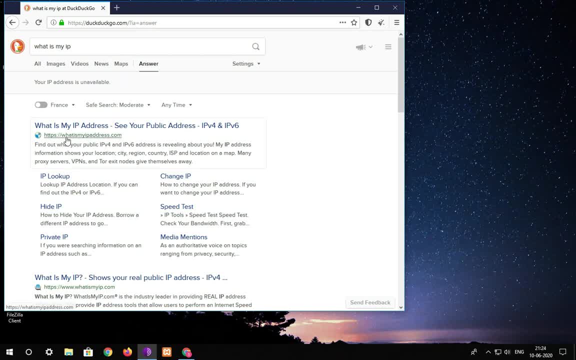 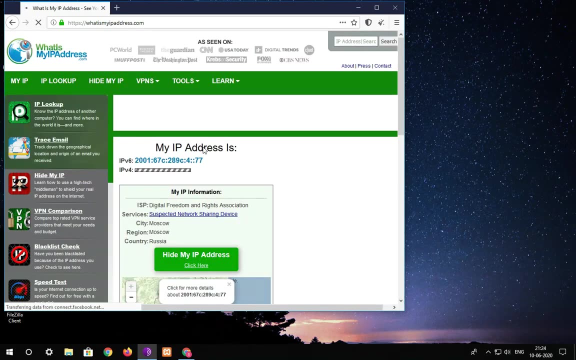 So okay, So this is the first site. What is my IP addresscom? So I'll just click on that first one. Okay, Fine, Come on my internet please, And, and, and. can you see this thing? 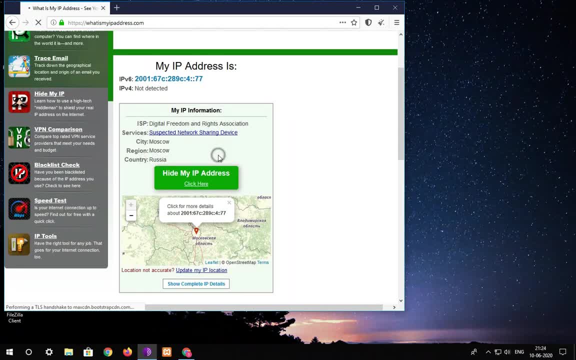 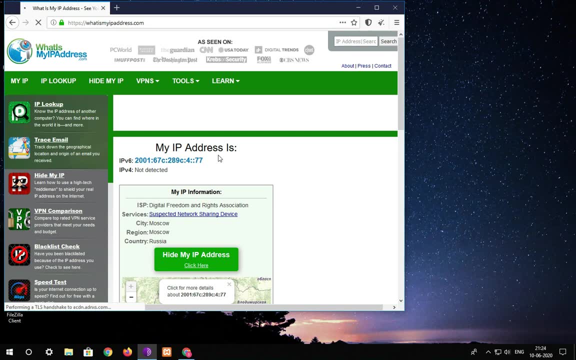 Moscow, Moscow, Russia. So what is this thing? What this thing actually means? It means that I am virtually connected to a network or a server which is set up in Russia or Moscow. I know you didn't understand what I said, but let me make this simple to you. 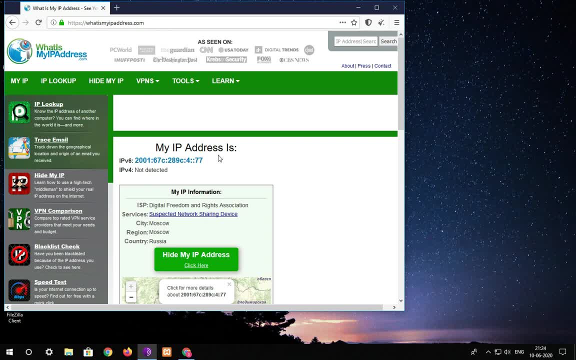 So what actually this is, this says is that you have actually connected to a virtual private network. Okay, But the thing is that you can also download any other software. So let's say you have a virtual private network and just go on saying that I'm anonymous. 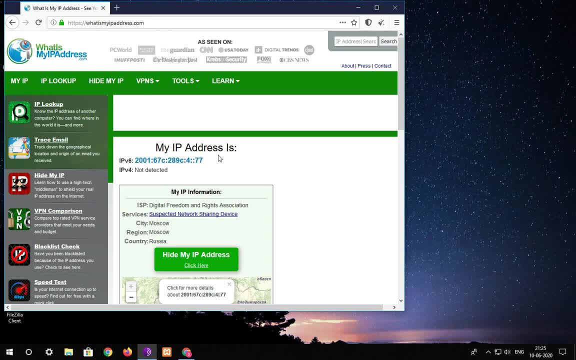 But the thing with Tor or the onion router is that it creates three links, or you can say three ports. Now, for example, this just shows that this is the Moscow which I'm connected to, But after Moscow, there are also two other layers which you are connected to. 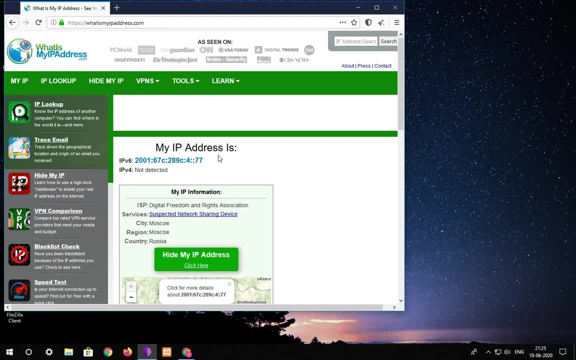 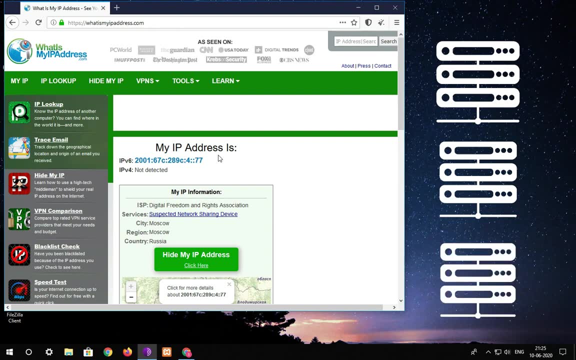 For example, you first connect to connect to a server like, let's say it's in France, The second one is in Australia And the third one will be Moscow. And the third and final one will only be the recognizable server, which others will be able. 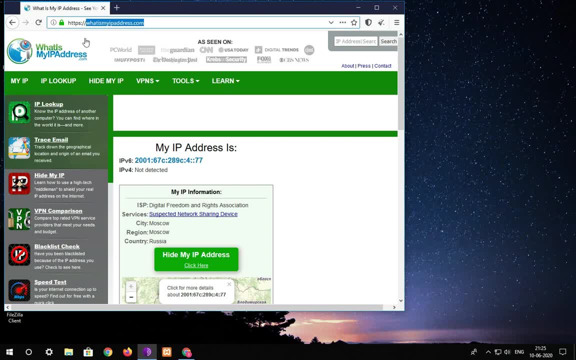 to see, For example, this server over here. or it says: what is my IP address, dot com. Well, this server or this website is just able to see the end server, or you can say the third server of your. like the connection Okay. 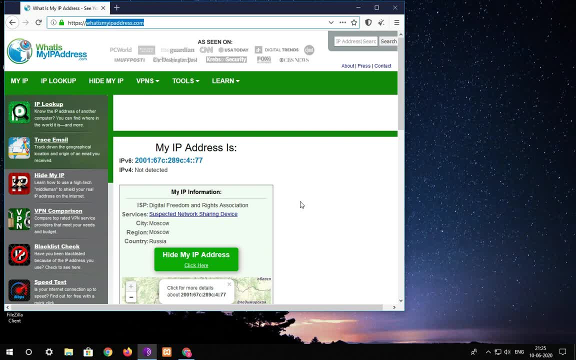 While the rest of the two, which is in my case, let's say, France and Australia, Let's say France and Australia- are undetected And along with that, my server, my computer, is also undetected. So that's the beauty of the onion router, which I really love. 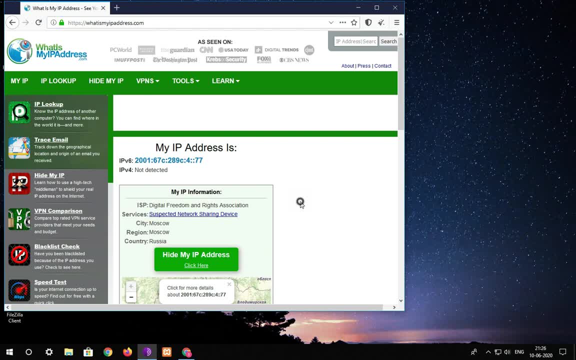 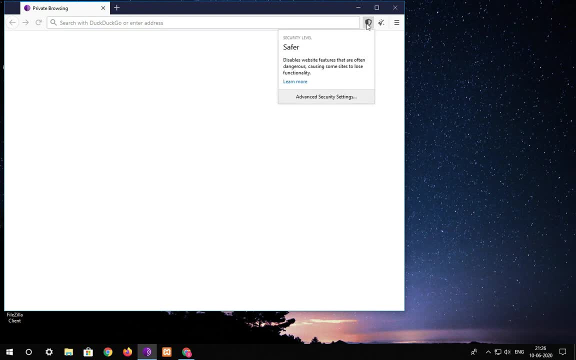 Okay, Now some people get tricks as well, which I want to share to you. Let me just close this thing. Okay, So there is this thing called as. you'll get this shield over here, So just go on and click in advanced security. 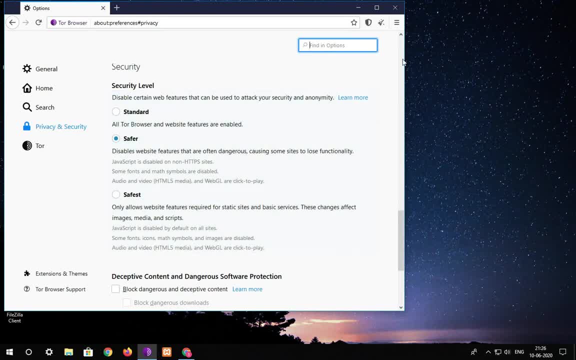 Okay, Now this shield actually says that. what should your browsing privacy or the security level be like? So I'll say that better, let it be on safer, because on standard it's like all the things will be visible and JavaScript and other hacking things will also be visible, which can make. 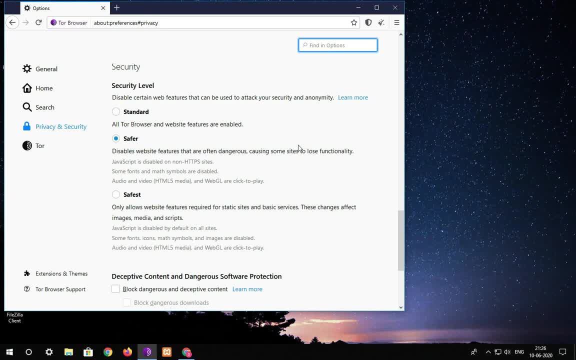 your computer like harmful and just. it will go like a zombie And the safest one will just block everything, which is really not good, Because if you want to access something, it will just say, hey, you can access this. It's not allowed over in here. 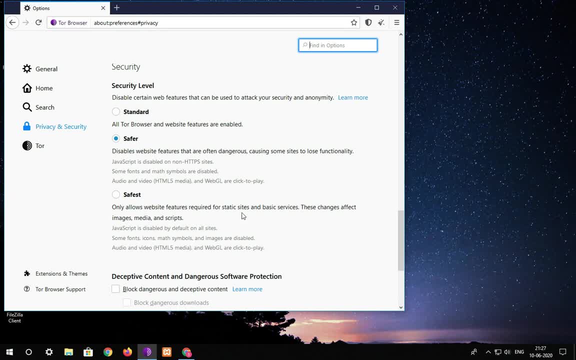 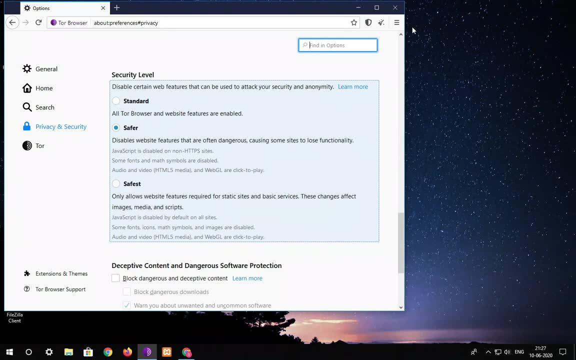 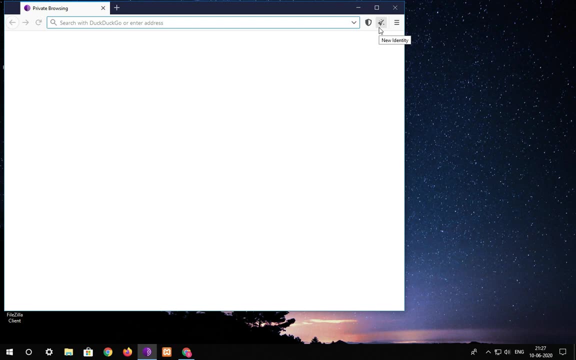 So that's why I just go on and select the safer option, which is really good, and you can just read all the features given over here. All right, So I'll just get back. Okay, Fine, I'll close this, And now the next thing which I want to show you is this: 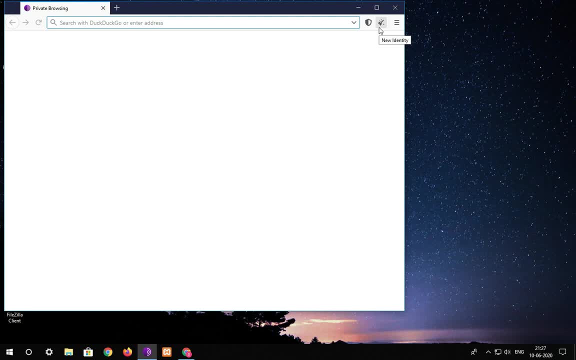 New identity. This thing really, really is amazing. Okay, So what does this thing actually do? Well, it says that it'll give you a new identity and just close all the browsers and like the tabs which you've opened, But the thing is that it gives you a new identity. 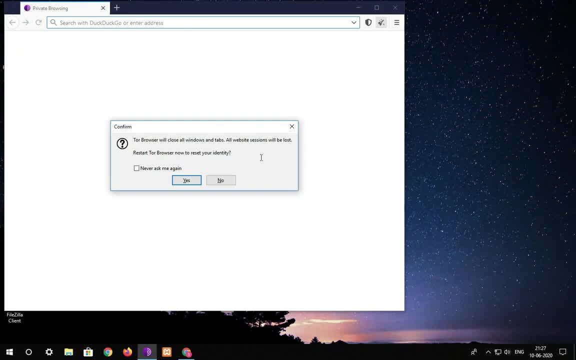 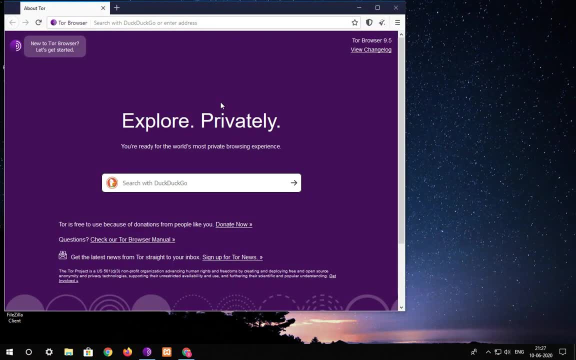 It means that, for example, currently I was connected to Russian server, Right, But when I just click on this thing like confirm, yes, It will connect me to a different server, or let's say a different like a server, Yes, Yes. 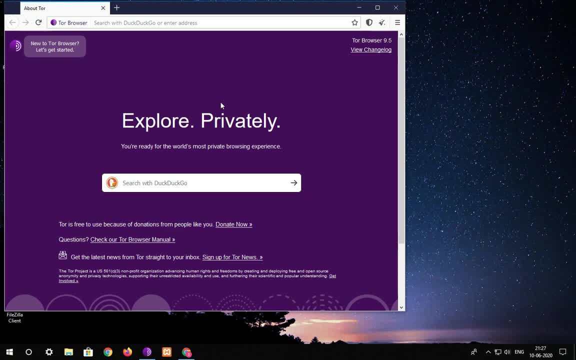 It's a server. It has to be a server, So it will connect me to a different server. All right, So now I won't give a demo of that, because I think the video is gone more than 13 minutes. 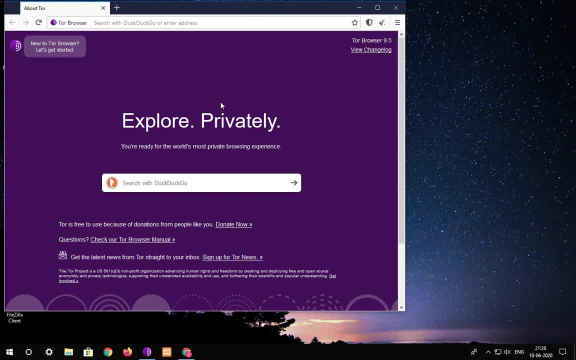 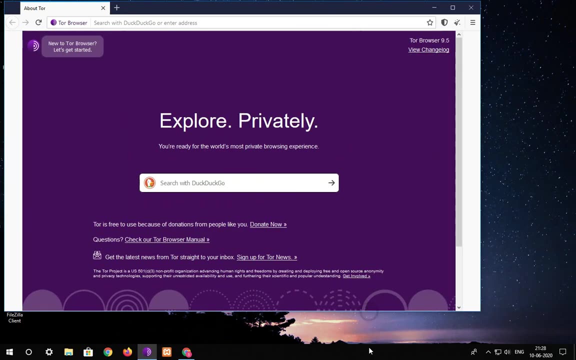 13 to 14 minutes, whatever. So I think this is the end of the video. But Before just ending of the video, let me tell you a good and a clear advice that please don't play with this, Okay. So just don't go this way, like horizontally and like this vertically.